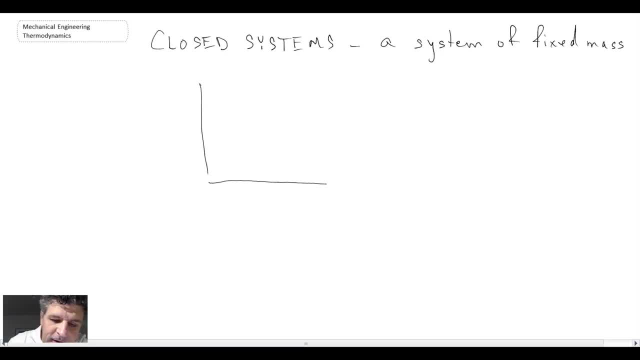 as an example, let's say we have a piston cylinder device, which is a very popular one that we'll use within thermodynamics, and if we have some stoppers here that are holding the piston at a given point, and let's put some weight on it so that provides a load, and within our cylinder let's imagine that 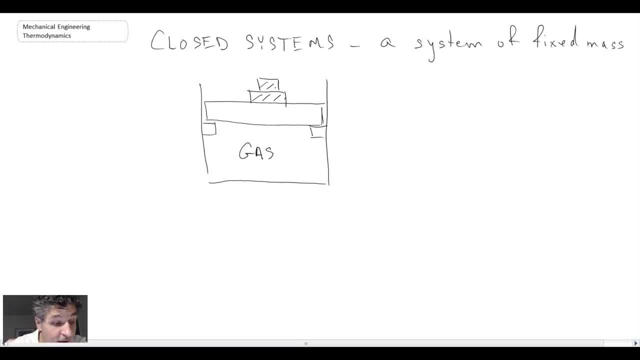 we have a gas Now what we will often do is we will draw a boundary around our system, so in this case the boundary would be along the walls of the cylinder and our gas is inside. Now we can have a couple of things that another term that we will have here will refer to that as being the boundary. 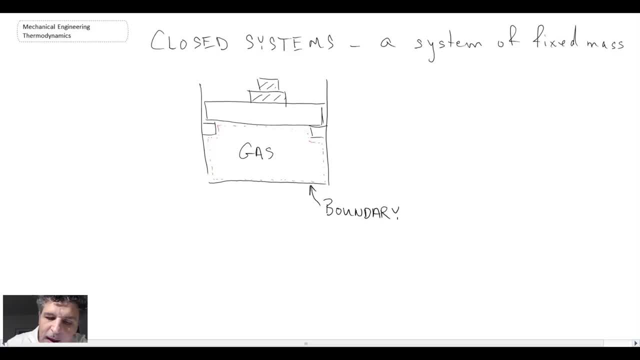 and out here, everything outside of our boundary we will refer to as being the surroundings. Now, with a closed system, you can have a couple of things crossing the boundary and those are the two things that are within the first law of thermodynamics for a closed system and, if you recall, we talked about 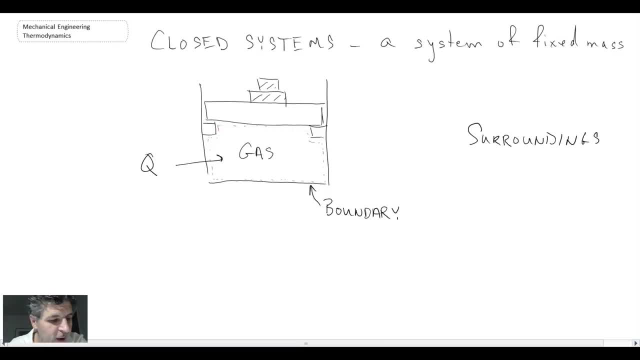 heat, so the capital Q and which work. Now, work can go either into or out of a certain system. In this case, what we will be doing is we'll be showing a schematic of putting work in, and we're going to do that with something. 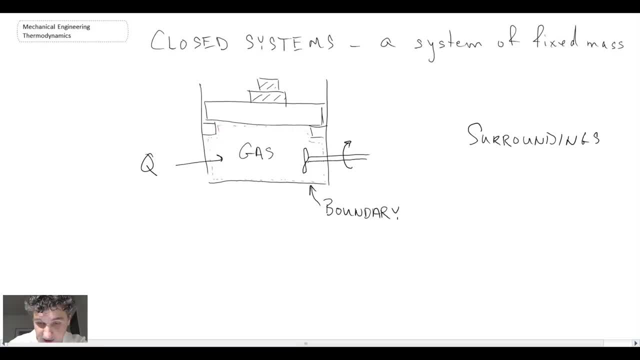 that is referred to as being shaft work. So we're rotating a propeller, in this case, which is inside of our system, and it would be heating up the gas on the inside And in the process. what we are doing is we're doing work and we've denoted that with a capital W, So in a closed system. 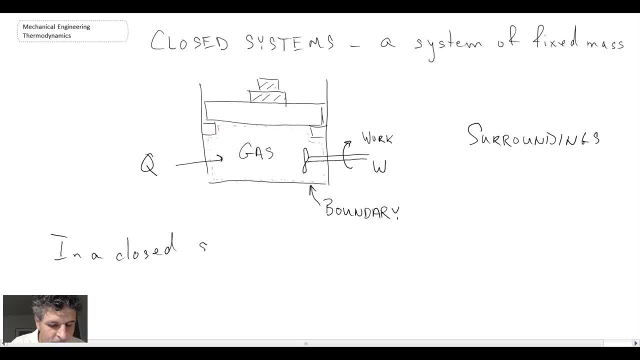 work and heat cross the system boundary. mass cannot, And that's why we call it a fixed mass system, So that is referred to as being a closed system. The second type of system that we will look at is the open system, And this is a system whereby mass can cross the boundary of the system. 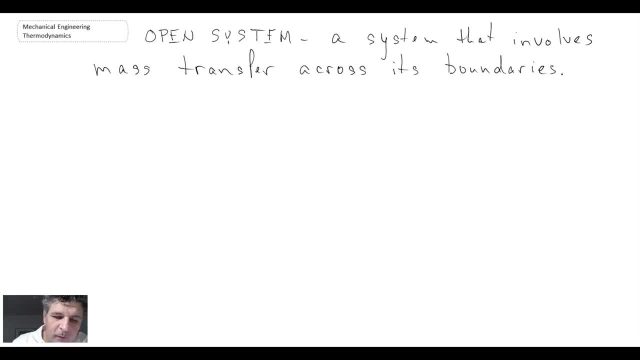 So to draw a schematic of an open system, let's say we have some inlet, we have some device that we have not defined, So this might be a turbo machine, for example, Such as a turbine or a compressor or a pump or anything like that. 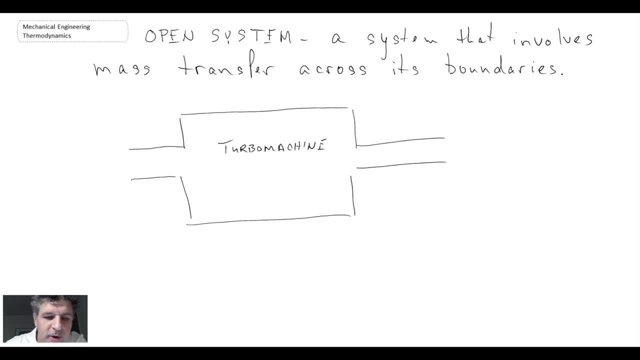 Just like this is a turbine or a 3.5 word compressor or a pump or anything like that. just like that goes everywhere. Just like with the fixed mass system, we have the boundary. here we're going to draw another boundary. however, this boundary is a little different because mass actually can cross. 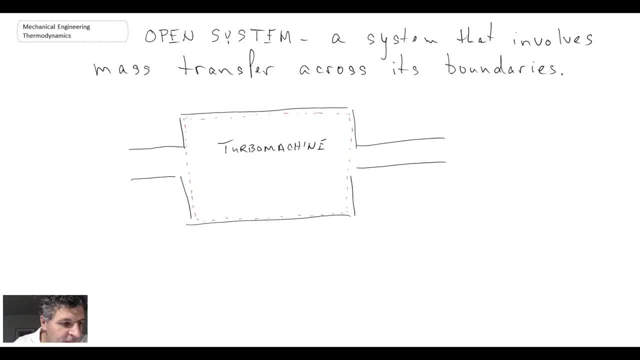 that boundary and we refer to that as being the control surface. and within the control surface, we sometimes refer to this as being the control volume. If you've taken a course in fluid mechanics, you have probably done control volume analysis by applying the momentum or the energy equation- very similar concept here. 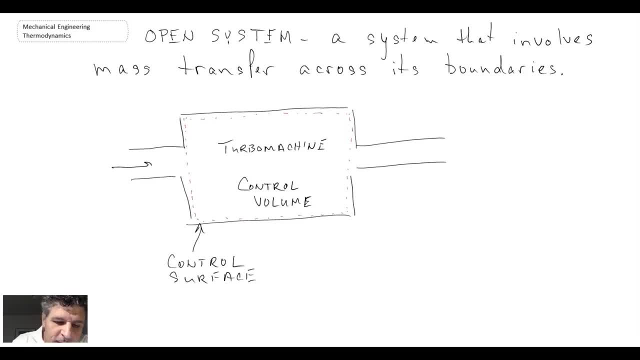 So what we have is we can have mass crossing the boundaries. so let's say we have mass flowing in and mass flowing out. What we will do is we're going to draw another boundary here and we're going to draw another boundary here and we're going to draw another boundary here and we're going to draw another.